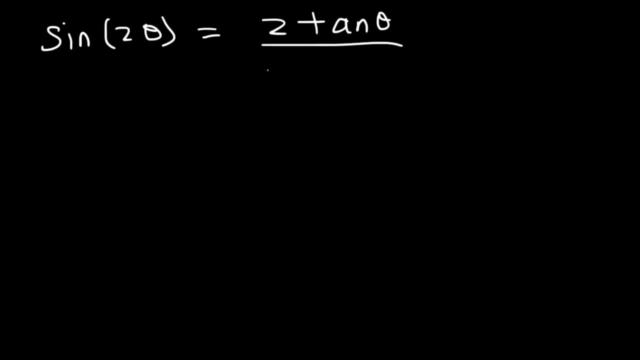 this is equal to 2 tangent theta divided by 1, plus tangent squared theta. So take a minute and work on this example. Sine 2 theta, we can use the double angle formula and convert it to 2 sine theta, cosine theta. If we look at all the angles of tangent it's theta And here this is 2 theta. So 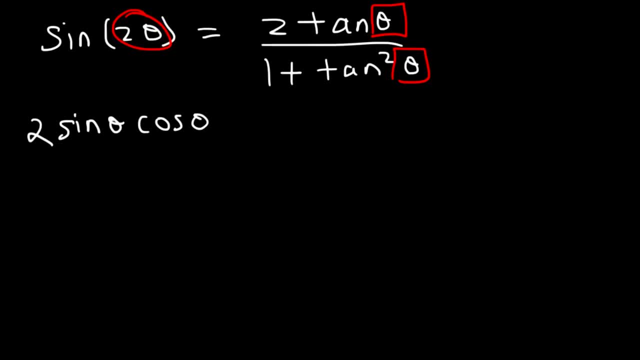 you've got to make sure the angles are the same first. So by using the double angle formula, we can take a 2 theta angle and break it down to theta. Now let's focus on the left side, So the right side is going to remain the same. I'm going to write this as: 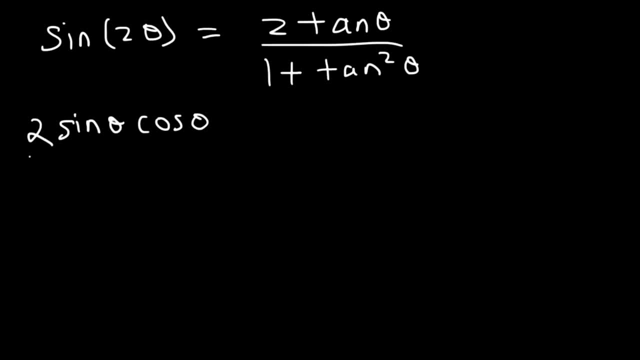 2 sine theta over 1.. And I'm going to multiply the top and the bottom by 1 over cosine squared. So what I now have is 2 sine theta, cosine theta and 1 over cosine squared. I'm going to write it as 1 over cosine theta times cosine theta. On the bottom I just have 1 over cosine. 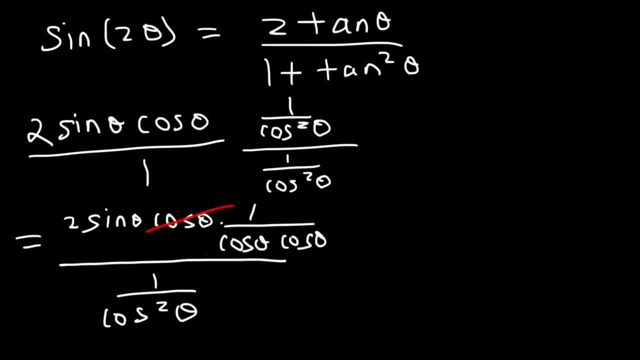 squared theta, One of the cosines will cancel, leaving behind one left over which I'm going to put under sine. So in the numerator I now have 2 sine theta divided by cosine theta And on the bottom I still have 1 over cosine squared. 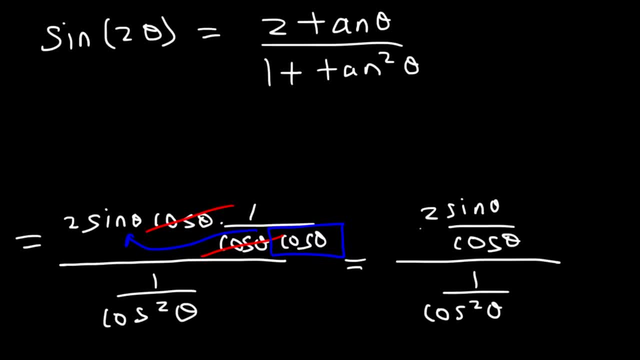 Sine theta divided by cosine theta is equal to what, Using the quotient identity, sine over cosine is tangent And 1 over cosine squared is secant squared And, if you recall, secant squared is 1 plus tangent squared. That's one of the Pythagorean identities that. 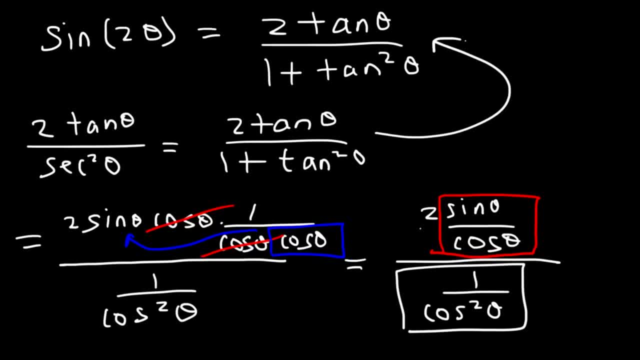 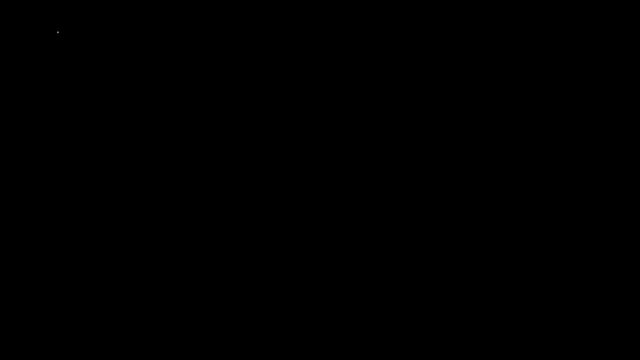 you need to keep in mind. So now we just showed how the left side is the same as the right side, So we've verified the identity. Let's show that 1 minus tan squared is equal to cosine 2x divided by cosine squared x. 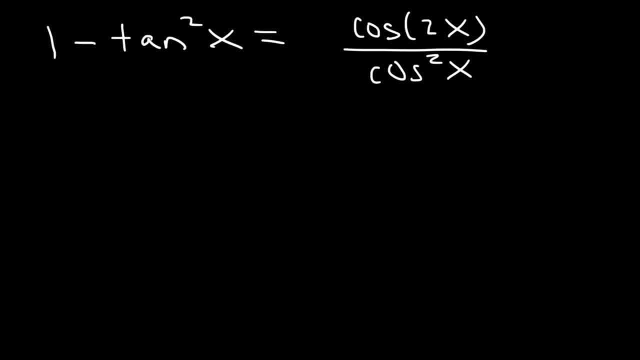 So how should we begin this problem? How can we take the expression on the left side and make it look like the one on the right side? Well, for one thing, we know that tangent is sine over cosine, So tan squared is the tangent over cosine squared, And the tangent 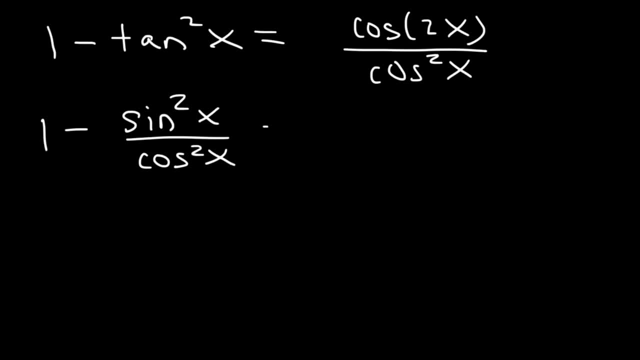 is the one on the right side, And this tangent is the tangent over cosine squared, And the is sine squared divided by cosine squared. So notice that we have a cosine squared on the bottom, which is what we want if we look at the right side. 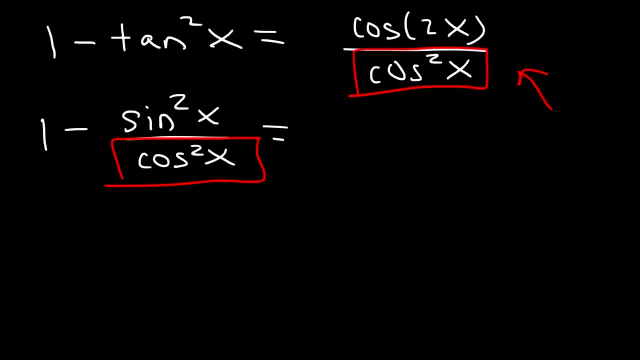 So we don't want to change the cosine squared. Now what we can do is multiply 1 by cosine squared over cosine squared. Cosine squared divided by cosine squared is 1. And the purpose for doing this is to get common denominators. 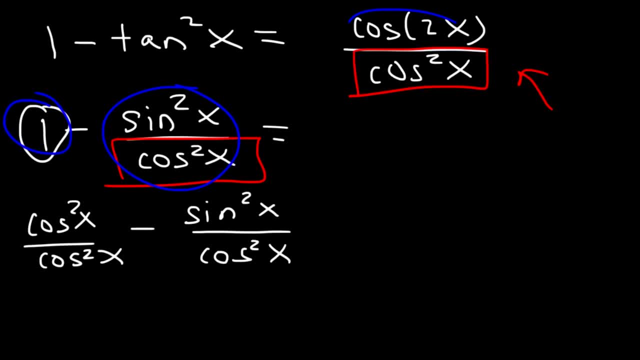 As you can see, we have two terms on the left and only one term on the right. So to go from a two-term expression to a one-term expression, we need to combine the two fractions into a single fraction. So to do that, it's going to be cosine squared minus sine squared, all divided by the common. 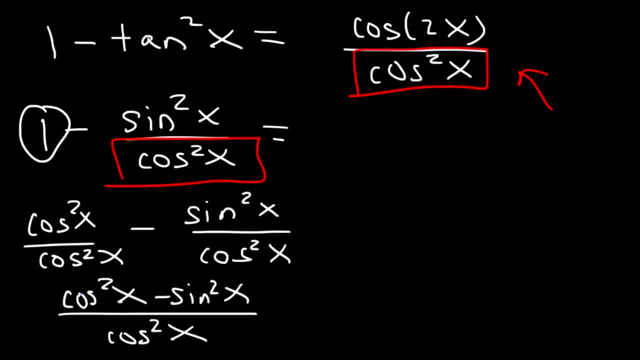 denominator of cosine squared. Now do you recognize this expression? Cosine squared minus sine squared is a double angle formula for cosine. It's cosine 2x. So now the left side appears just the same as the right side. so we've verified the identity. 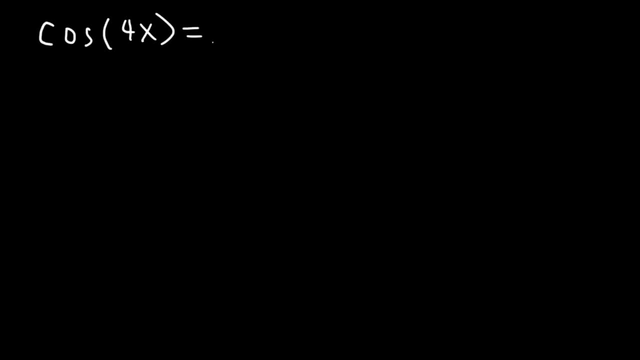 Go ahead and show that cosine 4x is equal to 8, cosine to the fourth power of x minus 8, cosine squared Plus 4x Plus 1.. So go ahead and work on this example. Now there are some special formulas for cosine you need to be aware of. 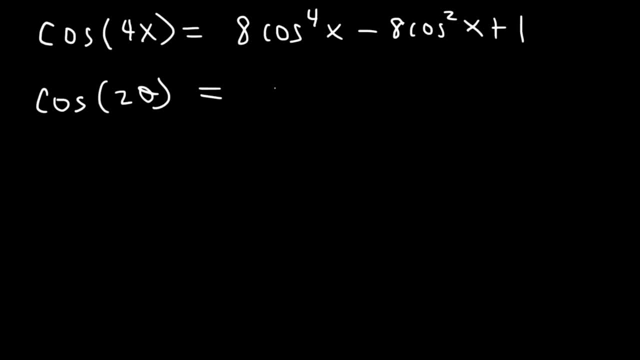 You know the first one: Cosine 2 theta is equal to cosine squared minus sine squared. So this is the double angle formula. but there's three versions. For instance, cosine squared is 1 minus sine squared. So therefore cosine 2 theta is equal to cosine squared minus sine squared. 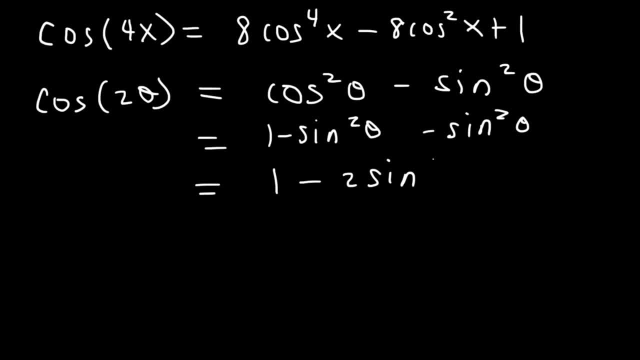 Cosine 2 theta is also equal to 1 minus 2 sine squared theta. So this is the first form that you want to be familiar with, and here is the second form. Now, going back from the first form, we can replace sine squared with 1 minus cosine squared. 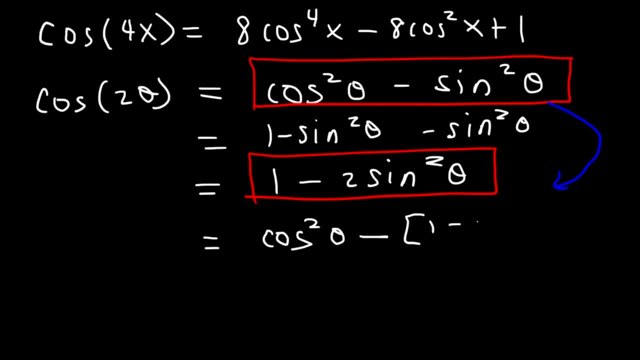 So we'll have cosine squared minus 1, minus cosine squared, And so that's going to be cosine squared minus 1.. Plus cosine squared, And so we'll get the other version of the double angle formula, which is 2 cosine squared minus 1.. 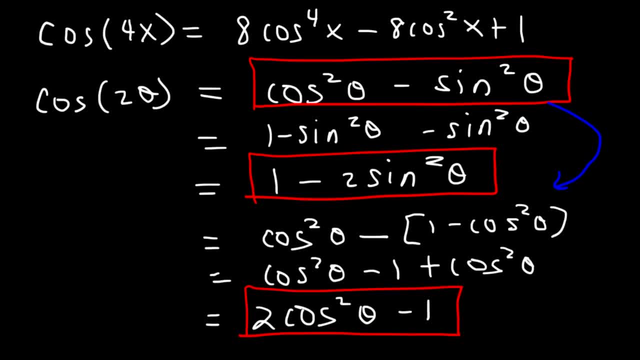 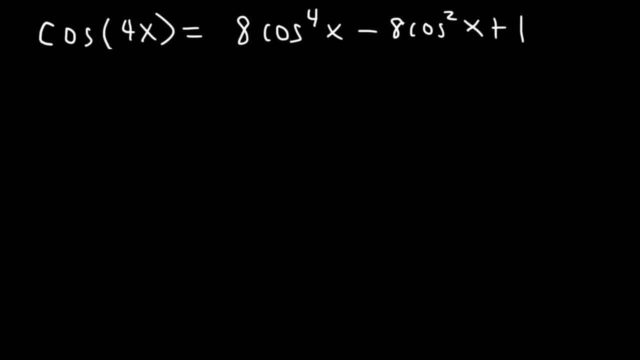 Now you want to be familiar with these three forms. So if we look at the right, everything is in terms of cosine. So we're going to use this form of the double angle formula of cosine in this particular example. Now, looking at this angle, we need to bring it down from 4x to 1x. 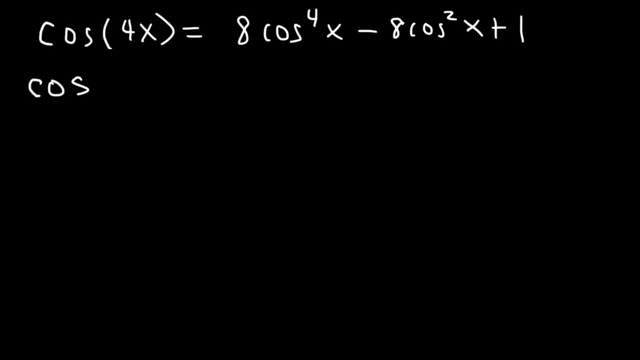 So you should always use the double angle formula if you want to reduce the angle from a large angle to a small angle, Anytime you want to cut it by half or even more. Now we know that cosine 2 theta is 2 cosine squared theta minus 1.. 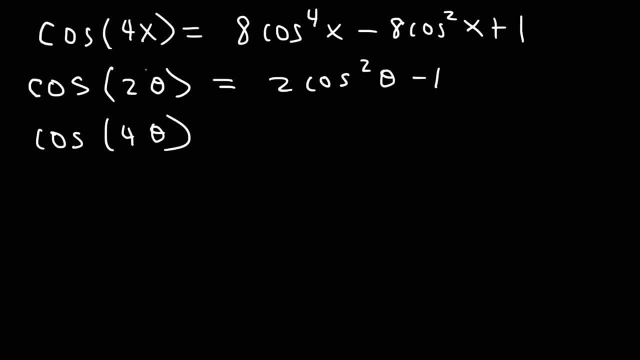 Now what about cosine 4 theta? Well, if we double 2 theta to 4 theta, we should double theta to 2 theta, So cosine 4.. 4 theta is 2 cosine squared 2 theta minus 1.. And so you can keep reducing the angle by half using the double angle formula of cosine. 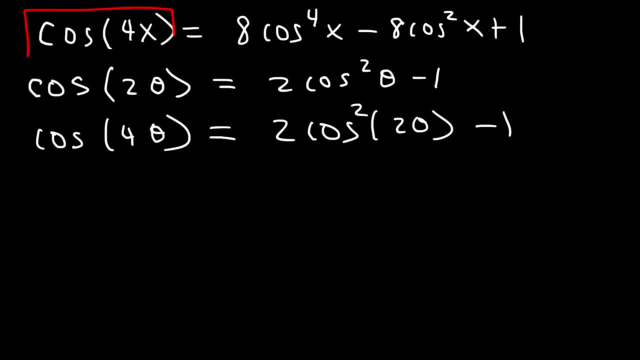 So let's replace cosine 4x with this expression in terms of x. So I'm going to put it here. So on the left side we now have 2 cosine squared, 2x minus 1.. I'm going to be rewriting. 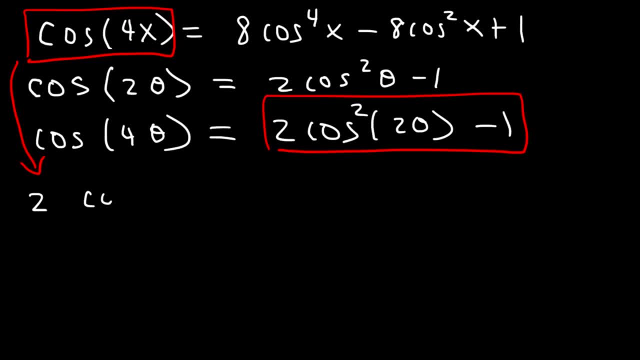 I'm going to rewrite that expression. So I'm going to rewrite it like this: 2 cosine 2x, And the cosine is squared, but I'm going to put the squared on the outside, Minus 1.. Now, the reason why I wrote it that way is because I'm going to use the double angle formula again. 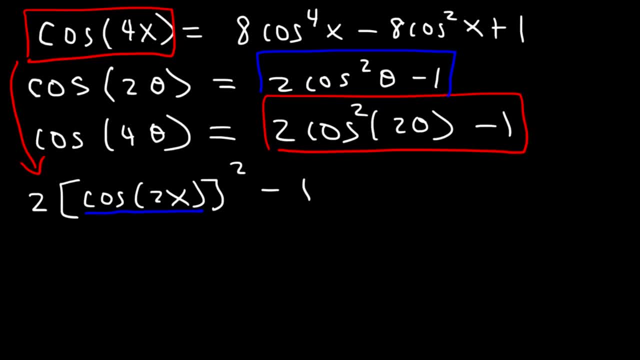 I'm going to replace cosine 2x with 2 cosine squared x minus 1.. So the first time you use the double angle formula, 4x gets reduced to 2x. But you need to do this. You need to do it again to bring 2x down to 1x. 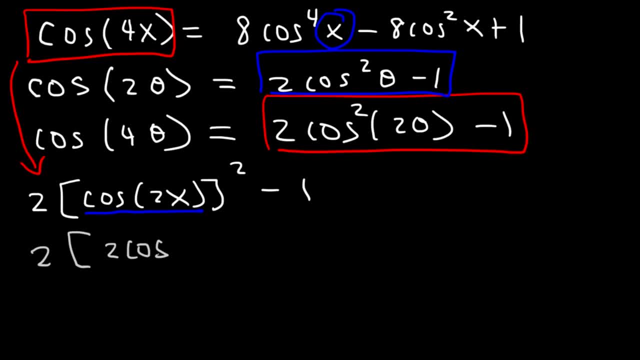 So this is going to be 2 cosine squared theta. Actually 2 cosine squared x minus 1, squared minus 1.. Now this expression, we need to FOIL it. So we have 2 times 2 cosine squared x minus 1.. 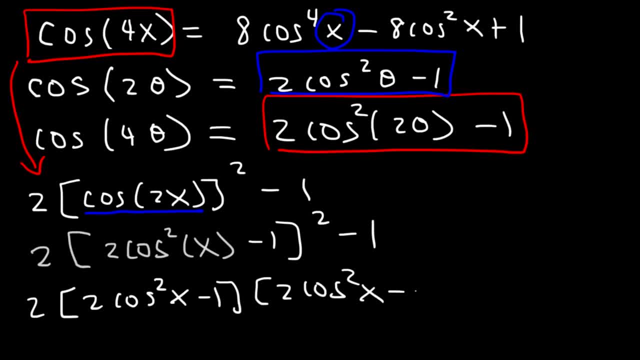 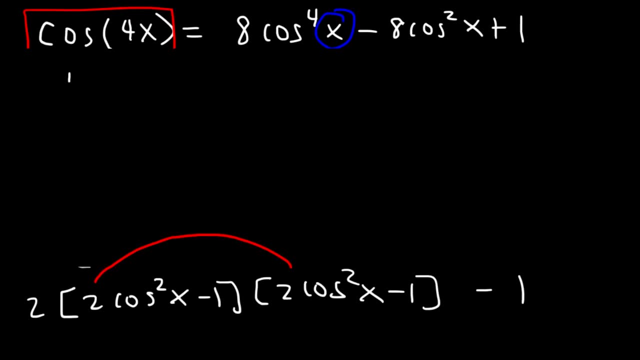 Times another 2 cosine squared x minus 1.. Minus 1 on the outside. Now let's FOIL 2 cosine squared times 2 cosine squared, That's 4 cosine to the 4th of x, And we still have a 2 on the outside. 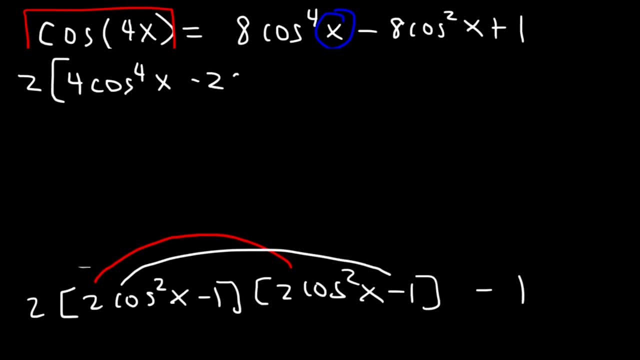 And then 2 cosine squared times negative 1.. That's negative 2 cosine squared. And then here we have negative 1 times 2 cosine squared, So that's going to be the same thing. And then negative 1 times negative 1, which is positive 1.. 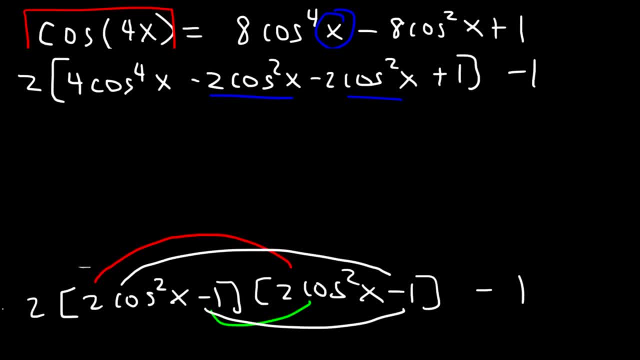 Next, let's combine like terms: Negative 2 minus 2 is negative 4.. Next let's distribute 2 to every term that we see here. So 2 times 4,, that's going to be 8. And 2 times negative 4,, that's negative 8.. 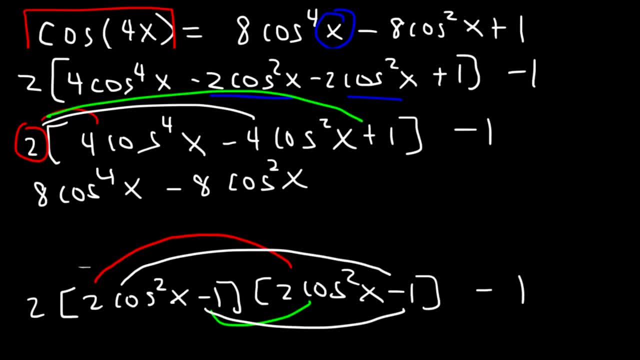 And then we have 2 times positive 1, which is positive 2.. And we also have the negative 1 on the outside. Now the last thing that we need to do is combine these two: 2 minus 1.. So our final answer is 8 cosine to the 4th power of x. 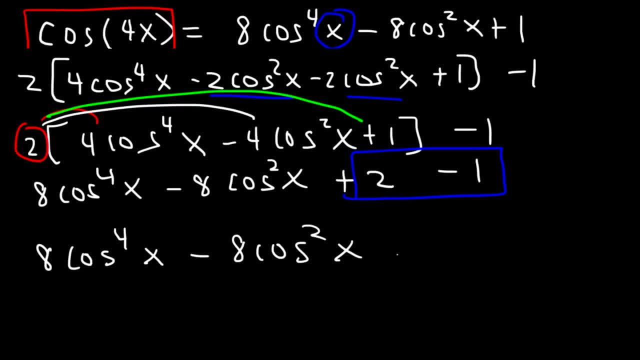 Minus 8 cosine squared, x Minus 8 cosine squared, And 2 minus 1 is positive 1.. And now the left side is the same as the right side. So that's how you can use double angle formulas to verify identities. 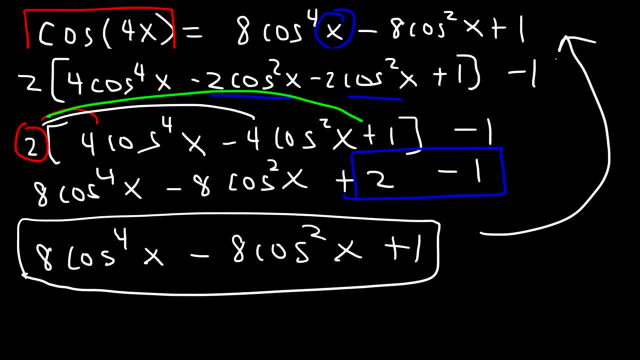 So anytime you want to bring an angle down, let's say from 4x to 2x to 1x, use the double angle formula. So if you want to bring it down from 2x to 1x, use it once. 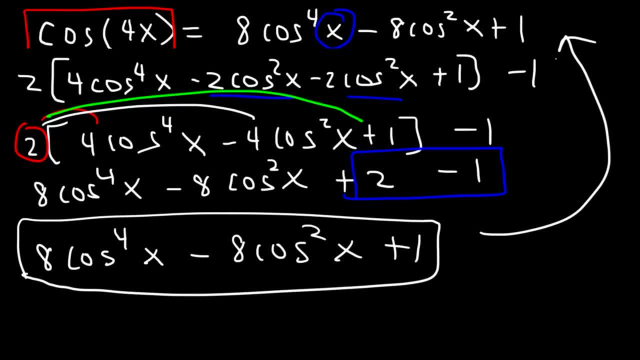 If you want to bring it down from 4x to 1x, you have to use it twice: 4x to 2x and then 2x to 1x. So if you want to bring it down from 8x to 1x, you need to use it three times. 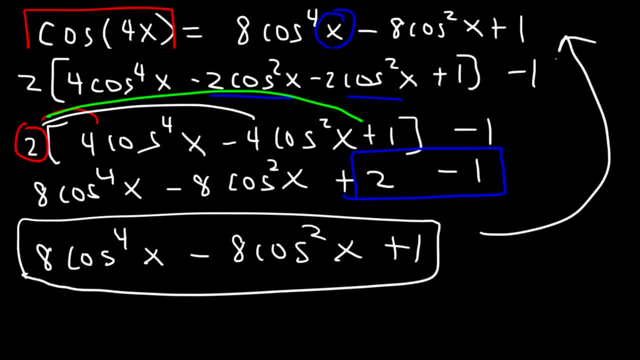 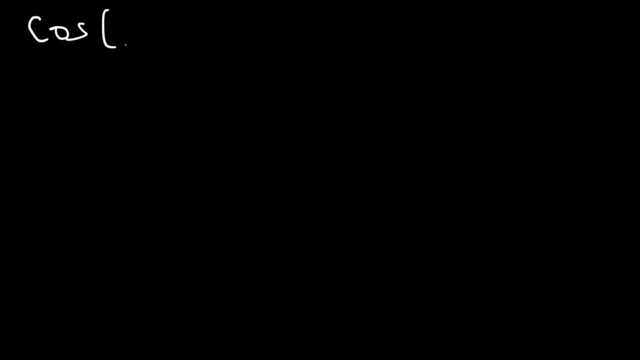 From 8x to 4x, that's the first time. 4x to 2x, that's the second time, And then 2x to 1x, that's the third time. Here's another one that we could try. 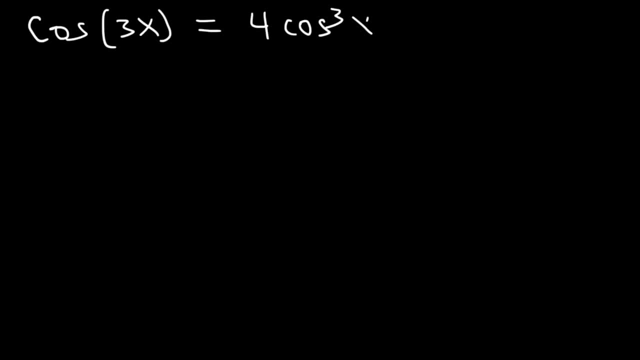 Let's show that cosine of 3x is equal to 4 cosine cubed x minus 3 cosine x. So how can we prove that? Well, we can. We can, We can prove that this equation is indeed true. Well, let's use this formula: 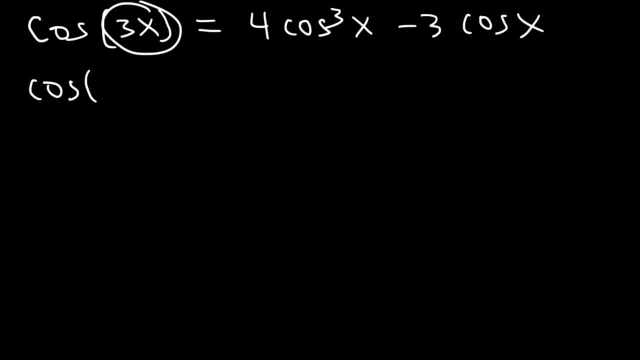 By the way, if you have an odd number, you can't use the double angle formula directly, Otherwise you'll get 1.5x. If you have an even number, like 4x or 8x, then you could use the double angle formula. 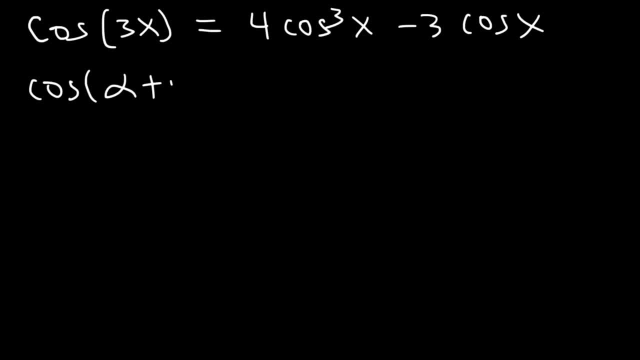 for cosine. But if it's odd, you want to use the sum and difference formula for cosine Cosine alpha plus beta. is cosine alpha, cosine, beta minus 4x to 2x. That's the first time. So cosine of 2x is cosine alpha, cosine, beta minus sine, alpha sine beta. 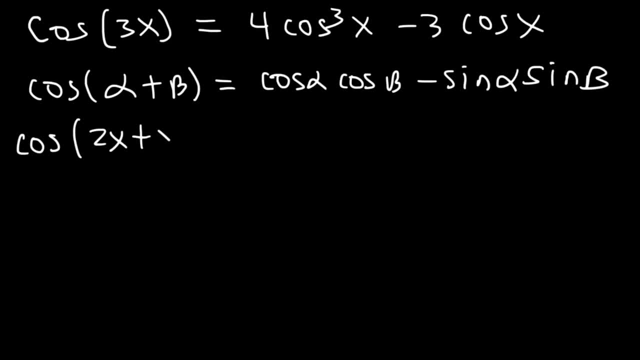 So 3x, we could say, is 2x plus x. So therefore alpha is represented by 2x and beta is represented by x. So then this becomes cosine of 2x multiplied by cosine of x minus sine of 2x. 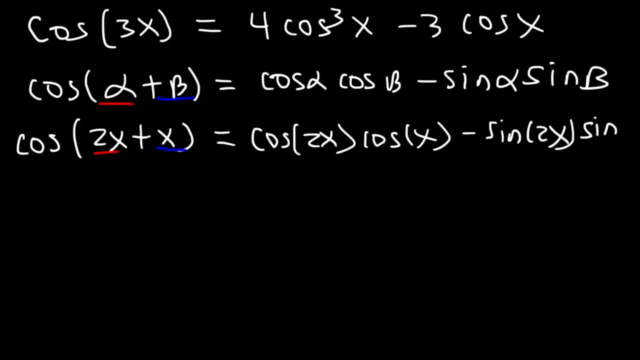 So all of that is equal to the original expression, cosine 3x. Now cosine 2x. we can use the double angle formula. Our goal is to convert all angles into x. So cosine 2x is equal to 2 cosine squared x minus 1.. 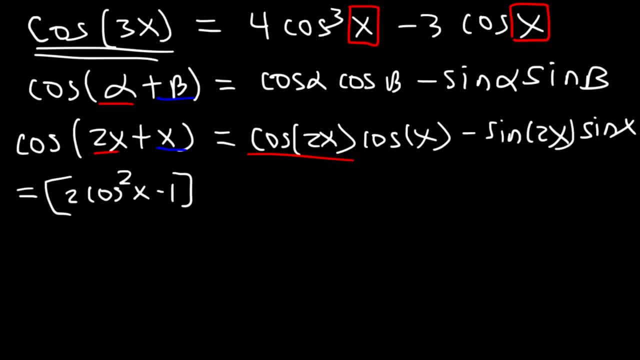 So that's one version of the double angle formula for cosine. We want to use that formula because everything on the right Is in terms of cosine, So every sine expression that we see, we need to convert it to cosine. Now let's get back to where we left off. 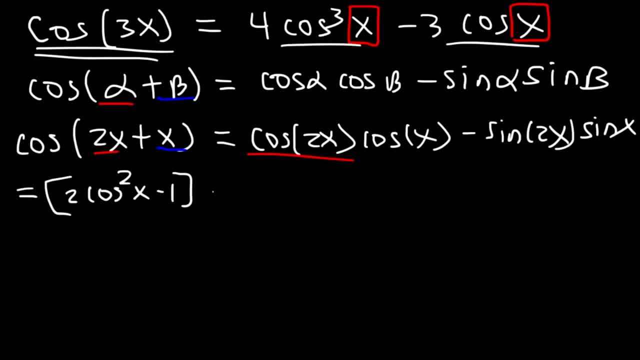 So these two are the same expression. So let's multiply 2 cosine squared minus 1 by cosine x, Now sine 2x, that's a double angle formula That's equal to 2 sine x cosine x, And we have another sine x attached to it.